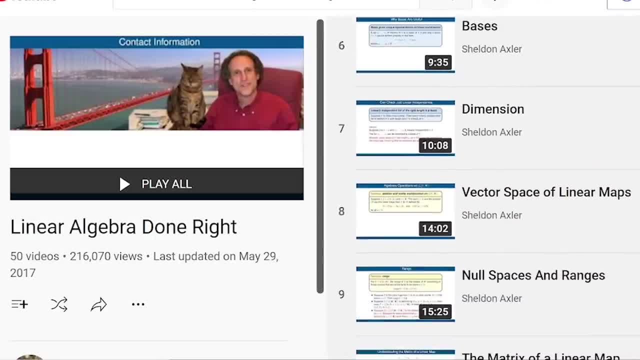 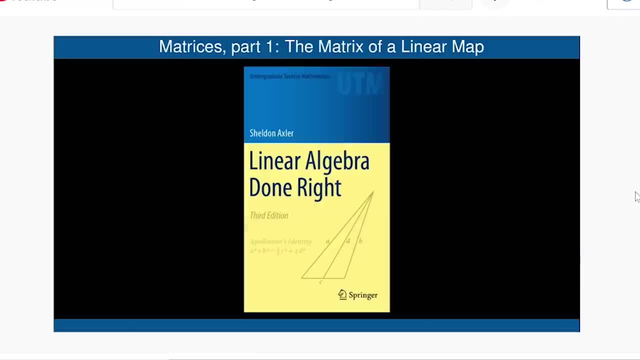 If you like videos, the author Sheldon Axler has made curated playlists just for this book, where for every concept in the book there is an associated video that explains that concept. 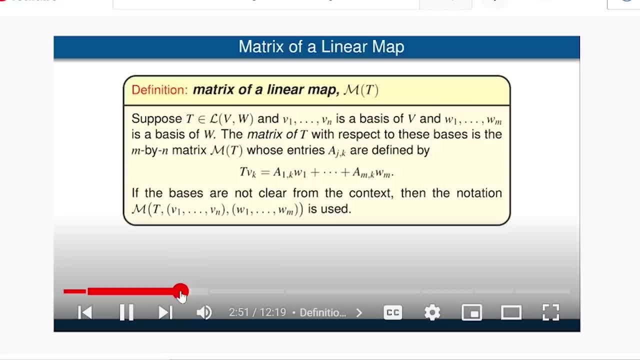 The videos are really short, and they're in bite-sized chunks, which makes them really nice for self-study. 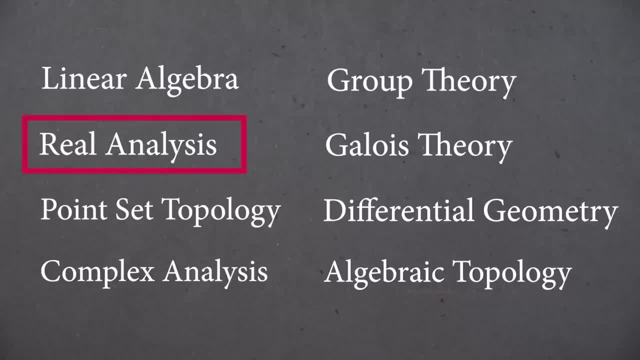 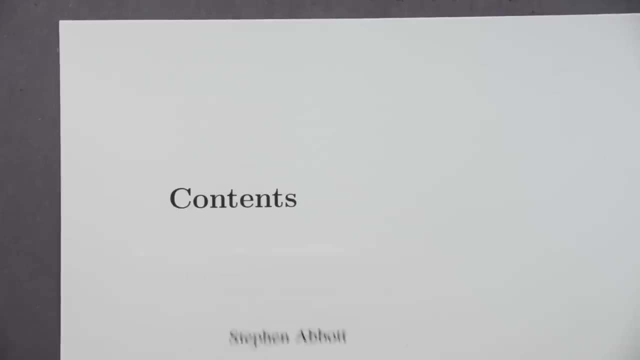 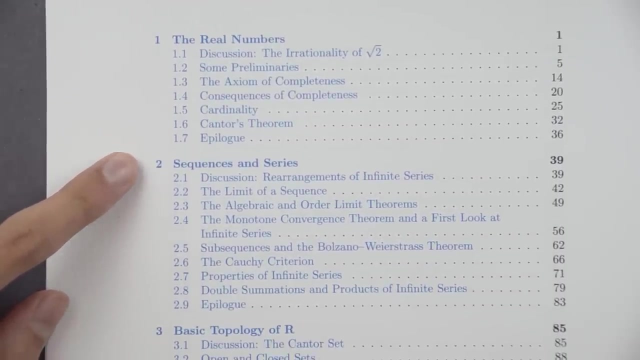 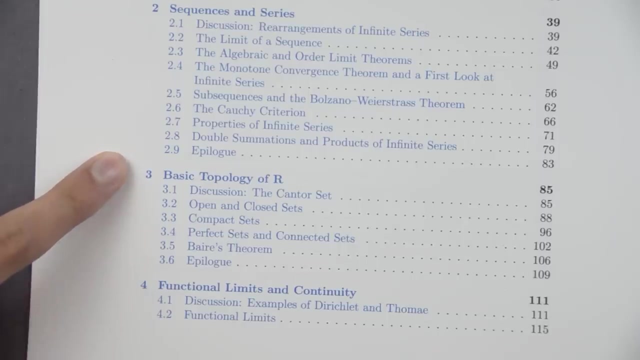 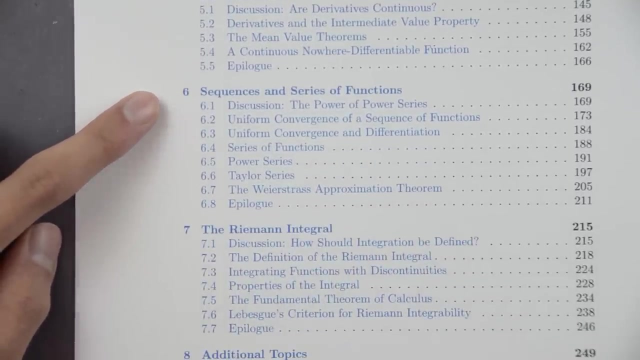 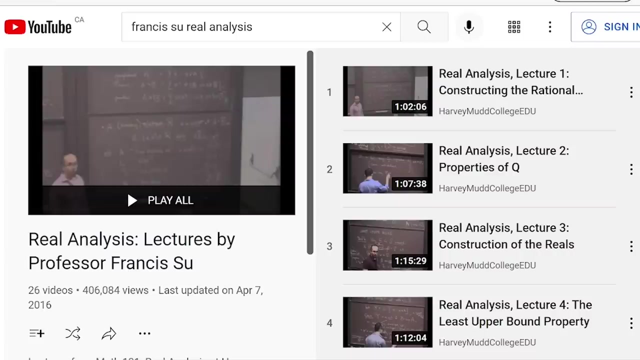 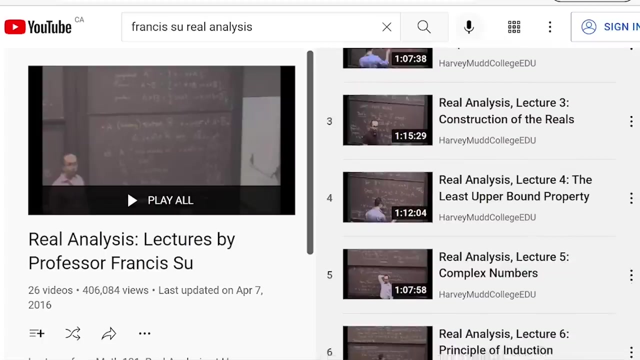 Next up is real analysis. Roughly speaking, this is calculus, but rigorously. You'll learn about epsilon-delta proofs, limits, derivatives, and integrals, all from a proof's perspective. The best book for learning this subject by far is Understanding Analysis by Stephen Abbott. So looking at the table of contents, it starts out by introducing the real numbers. It then talks about sequences and series, which introduces the language of analysis in a familiar setting. Then it goes into the basic topology of the real number line. And then calculus proper begins. Limits and continuity. And then derivatives. Then sequences and series of functions. And the integral. If you'd like videos, there's a YouTube playlist full of lectures by Francis Hsu, which is one of the most amazing lecture series I've ever seen on YouTube. They are so clear, and the professor is really, really empathetic towards its students. 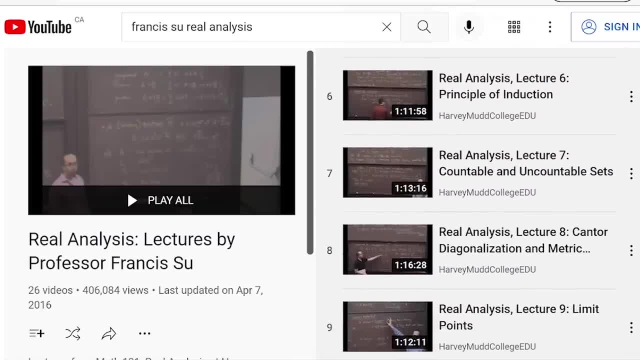 So you really feel like the professor is talking to you when you're learning the subject. 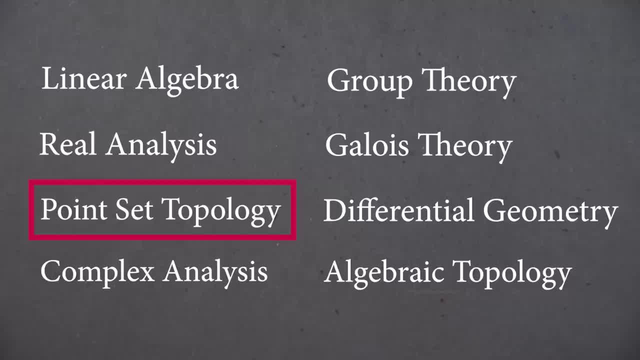 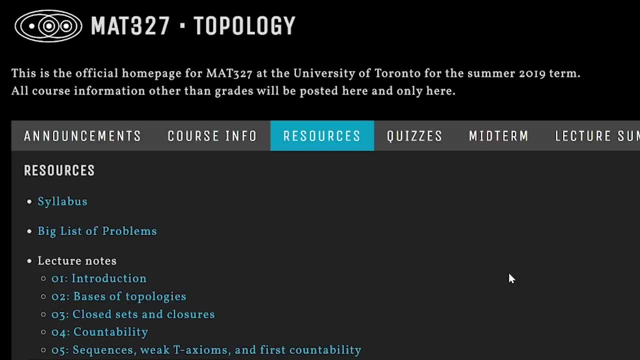 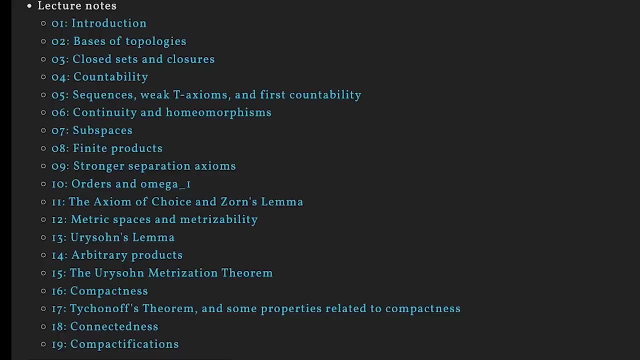 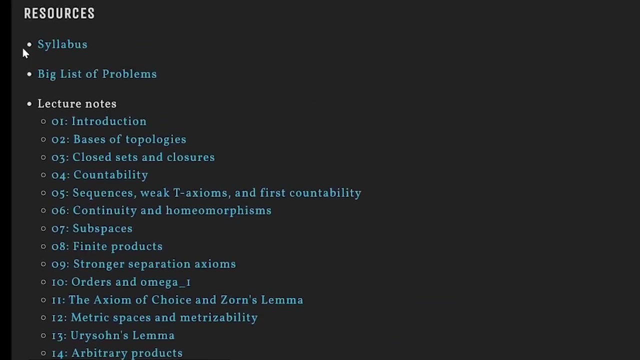 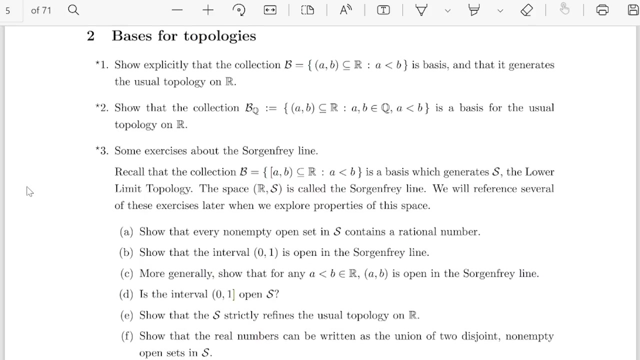 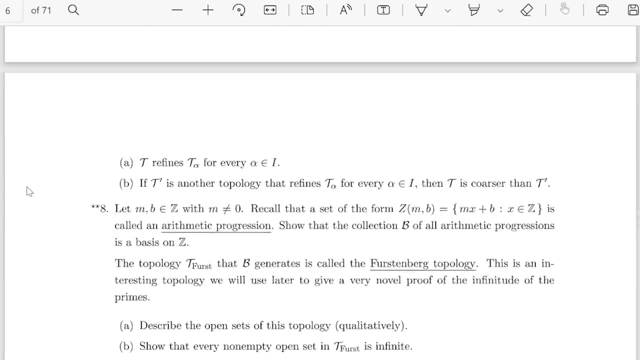 Next up on the list is point-set topology. This subject is about taking concepts from calculus and linear algebra, and putting them in a more abstract and general context. An amazing place to learn this is these online notes from the University of Toronto. For every single concept, there's a separate set of notes, which explain the concept with a lot of examples and motivation. There's also a gigantic list of problems, which is appropriately called the Big List. When I took this course at the University of Toronto, I went through this list and did every single problem. No joke. It took a lot of time, but it was immensely worth it. These problems are so illuminating, and anyone who does them all will come away with an incredibly strong understanding of the subject. 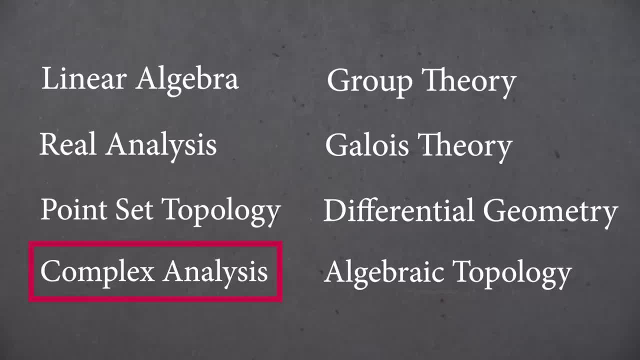 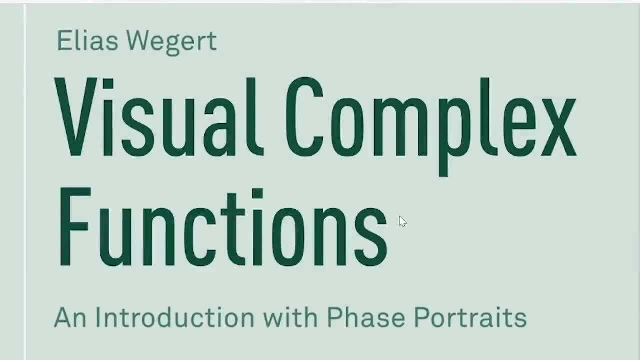 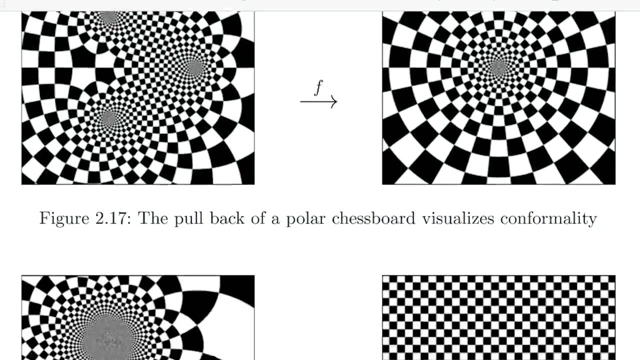 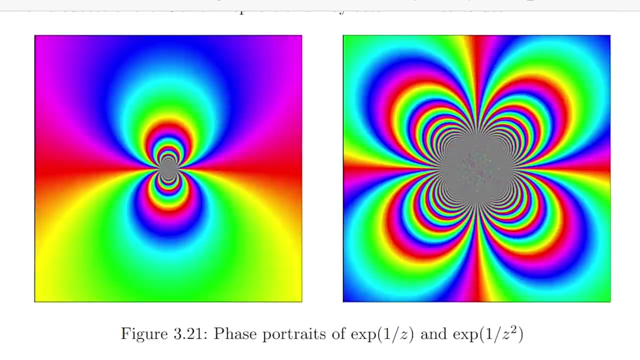 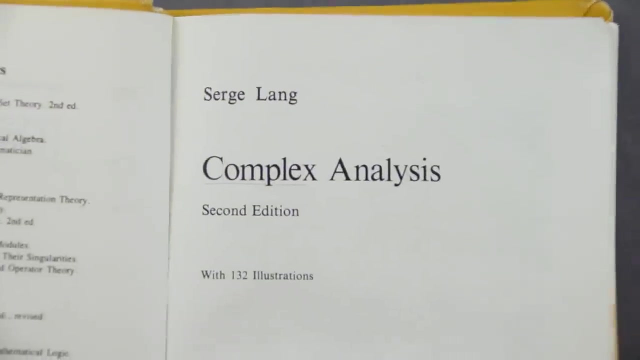 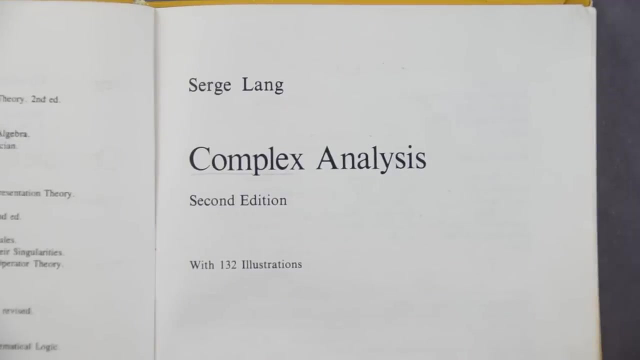 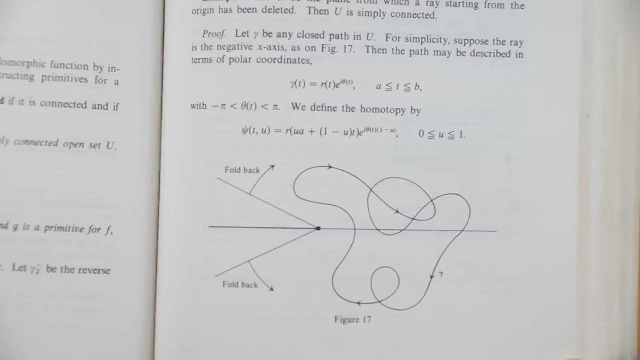 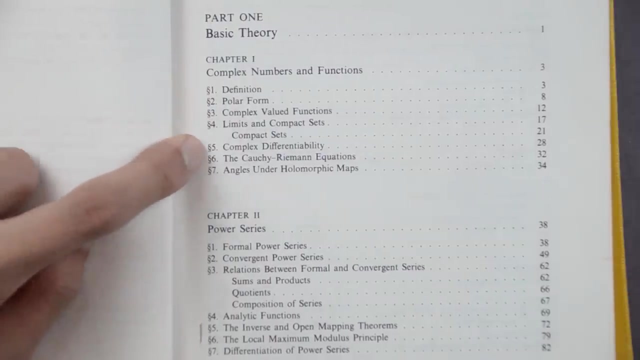 Next up is complex analysis. This is very roughly calculus, but with complex numbers. By far the best place to get an introduction for the topic is the book Visual Complex Functions, An Introduction with Phase Portraits. This is by far one of the most beautiful books I have ever read. It uses color and phase plots to illustrate the core ideas of complex analysis. The pictures are just so beautiful, and it's a great way to get a feel for complex functions before diving into the technical details. If you really want to get into the details, the book Complex Analysis by Serge Lang is quite good. And as a plus, it has 132 illustrations because somebody actually counted. What I love about this book is that it has tons of nice pictures. So it gives a wonderful geometric intuition for the subject. It also just makes it really fun to learn. So looking at the table of contents, it starts with the basic definitions. So what complex numbers are, and the basics of how to do calculus with them. The second chapter is about power series with complex functions. 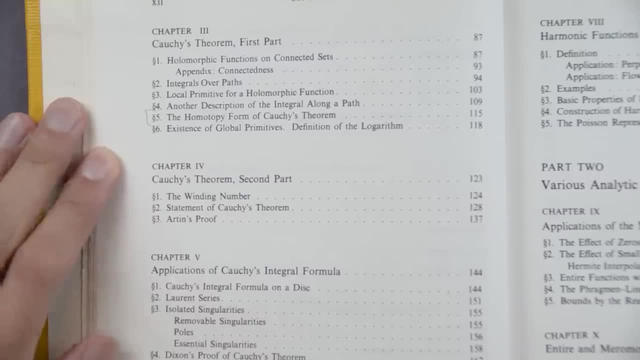 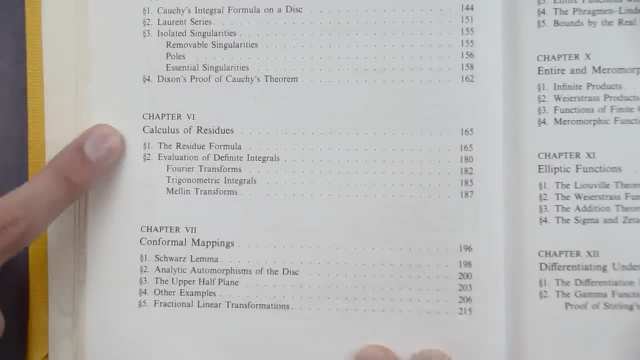 And then the fun begins. Integration in the complex plane. So here there are two big theorems. The first is Cauchy's theorem, which has two parts. And the second is the residue theorem. 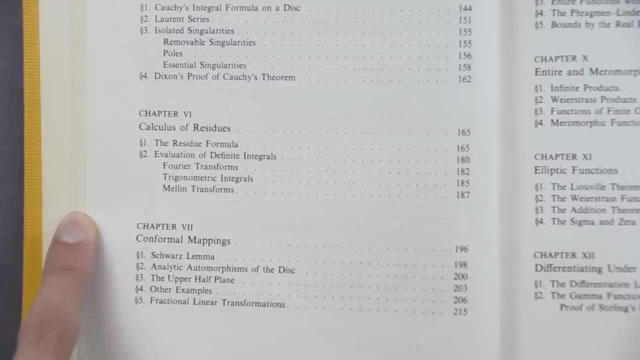 Up to this point is the contents of a first complex. So here there are two big theorems. The first is Cauchy's theorem, which has two parts. And the second is Cauchy's theorem, which has two parts. And the second is Cauchy's theorem, which has two parts. And the second is Cauchy's theorem, which has two parts. The rest of it is more specialized. It's very interesting, but it's not strictly necessary to understand the core of the subject. 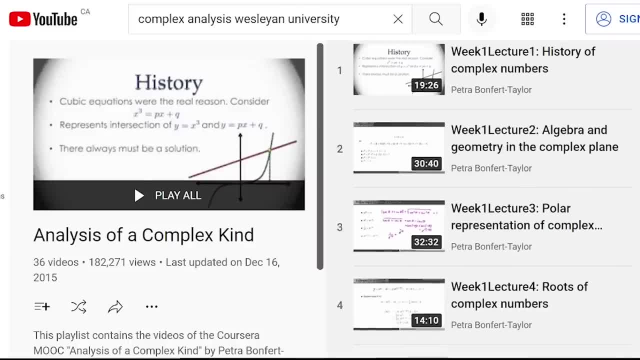 If you're more of a video person, you might like watching this playlist from Wesleyan University about complex analysis. All the links are in the description. 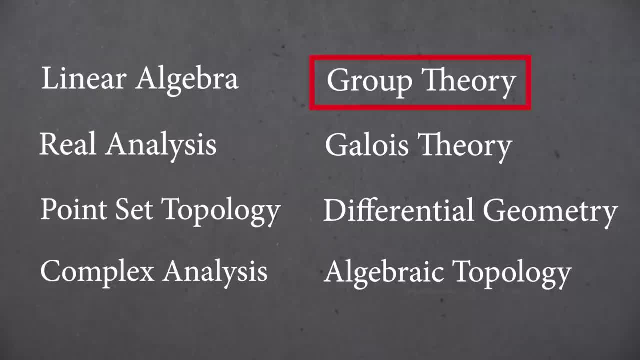 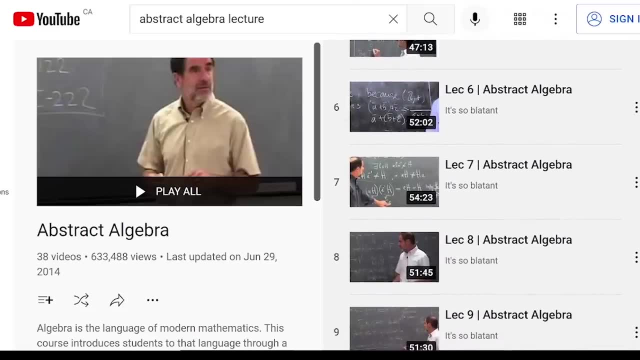 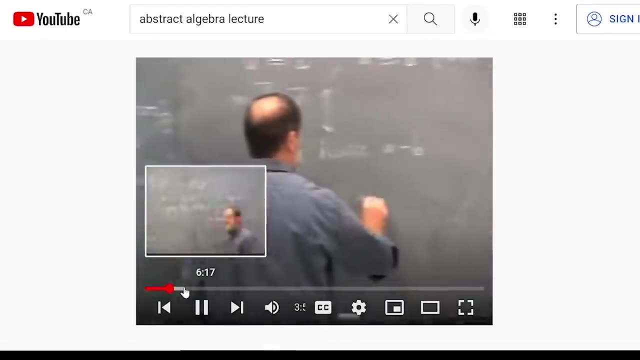 Next up, group theory. Roughly speaking, group theory is the study of symmetry. By far, the best place to learn the subject is these lectures by Professor Benedict Gross. These lectures are so clear and understandable, and Professor Gross is just so good at explaining ideas in an engaging and gripping way. 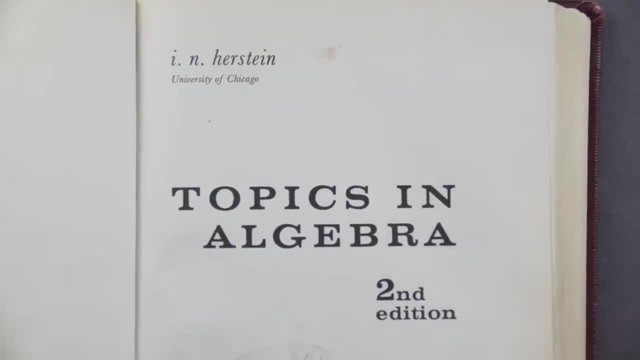 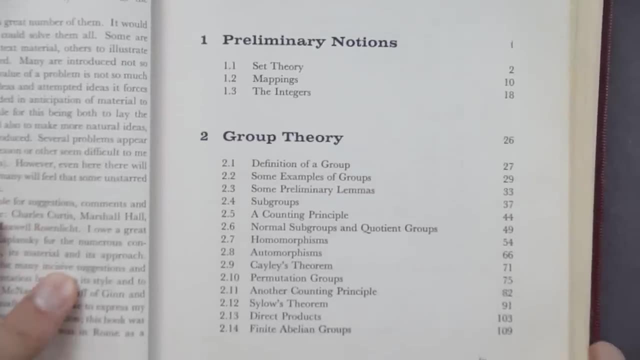 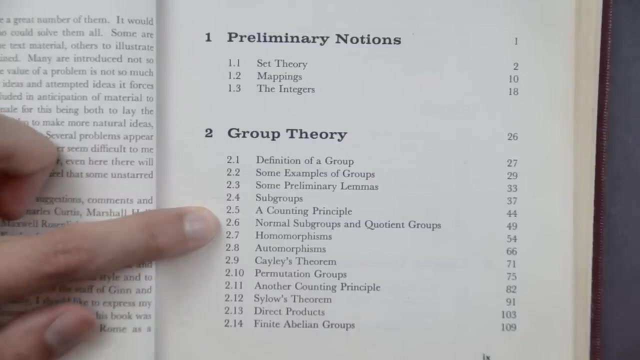 If you're into books, you might want to check out the book Topics in Algebra by Herstein. So looking at the table of contents, the part about group theory isn't the whole book, but it's just chapter two. It first introduces the basic definitions. What is a group? Then it talks about subgroups and quotients, two ways to build groups out of other groups. 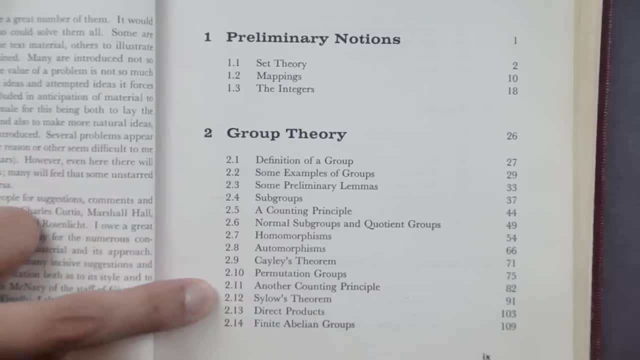 And it culminates with the two big theorems of group theory, the so-called Sylow theorems and the fundamental theorem of finite abelian groups. 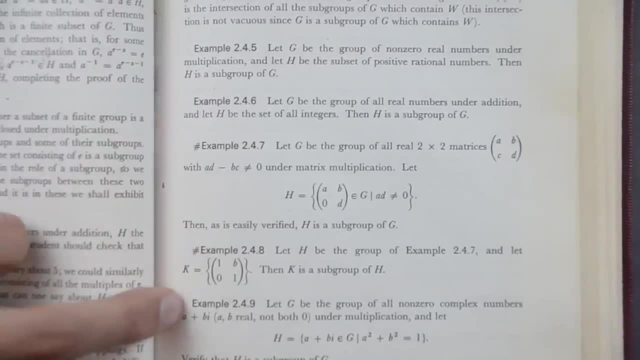 What I love about this book is that there are lots of examples, which makes it really nice for self-study. And at the end of each chapter, there is a truly gigantic list of exercises. Up next is Galois theory. 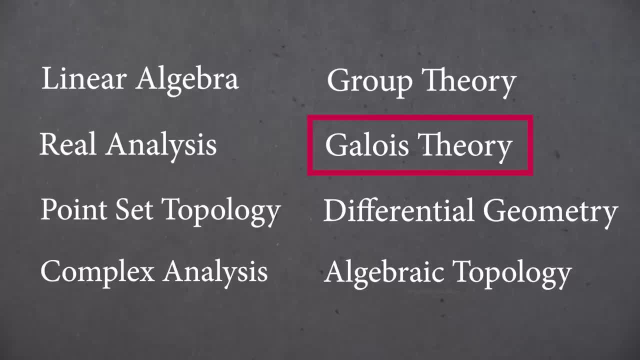 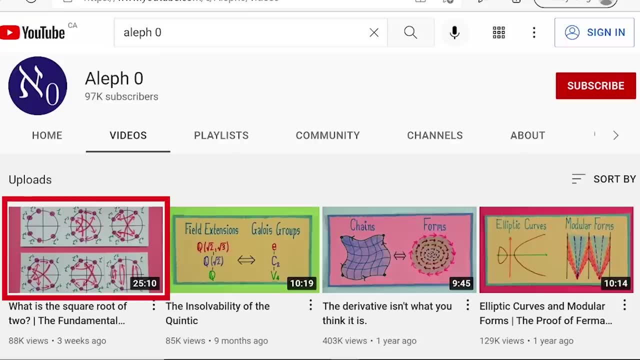 This is where group theory is applied to show that polynomials of degree five and higher don't have a general formula in radicals. Now there's a video on this channel that gives an introduction to the subject if you'd like to dip your toes in. 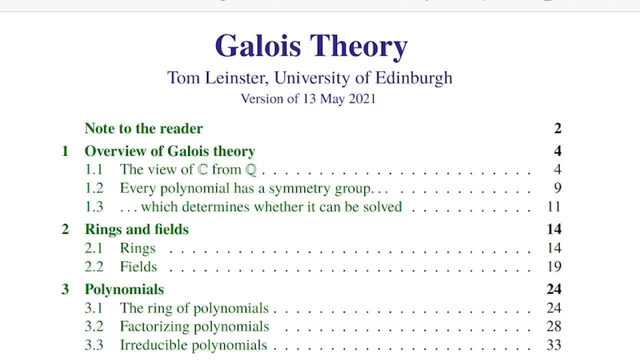 For a more in-depth explanation, these notes by Professor Tom Leinster are just amazing. They are freely available on the internet, and they are so understandable. 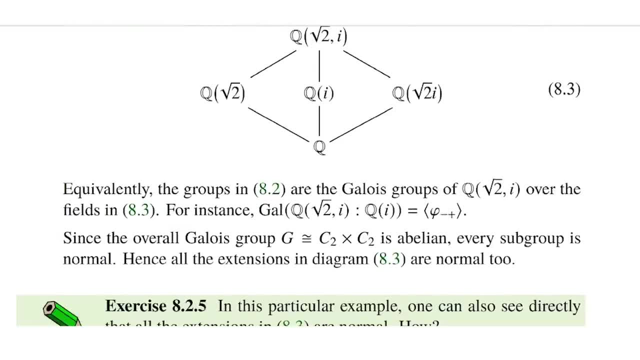 They have lots of exercises and examples throughout, which makes them really good for self-study. 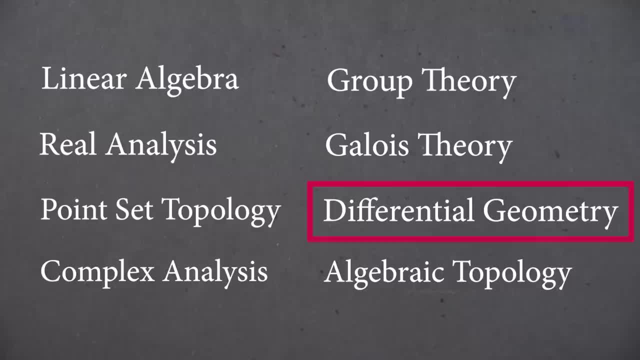 Up next is Differential Geometry. This is the study of curved surfaces in higher dimensional space, called manifolds. 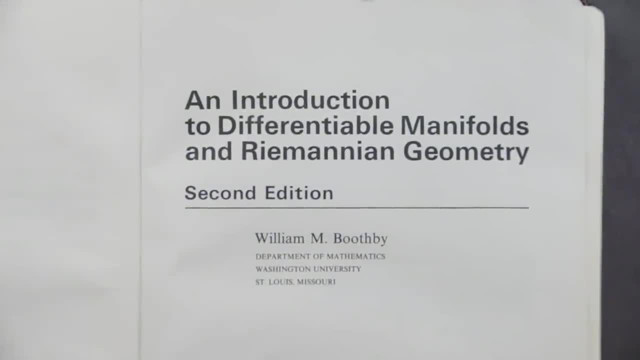 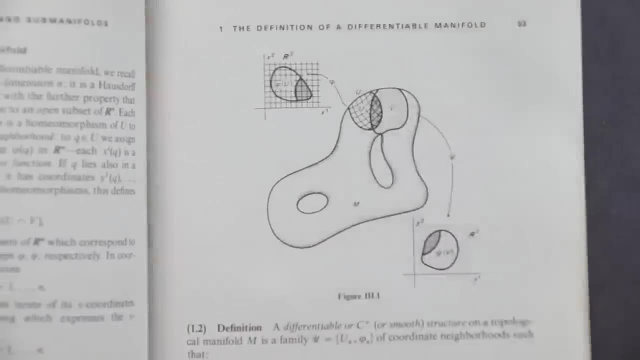 A wonderful book to learn the subject is the book Introduction to Differentiable Manifolds and Riemannian Geometry. This book is completely rigorous, but it also has lots of pictures and intuitive discussions, which makes it really fun to read. 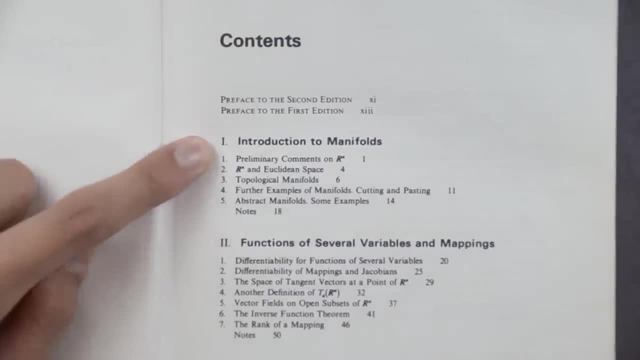 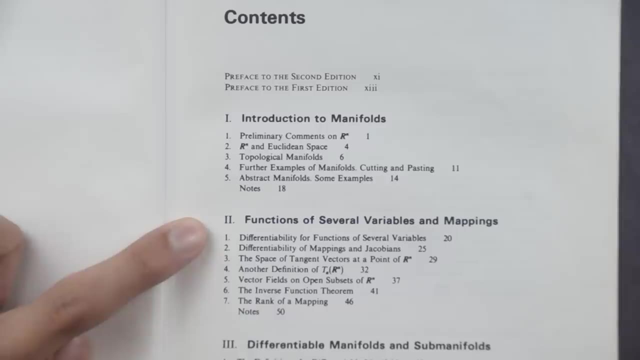 So looking at the table of contents, it starts out with an informal introduction to what manifolds are. It then talks about calculus in n-dimensional space, which is a prerequisite to knowing how to do calculus on curved surfaces. Then it introduces what manifolds are properly. 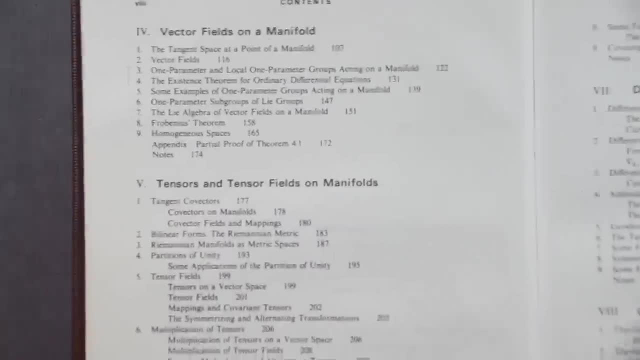 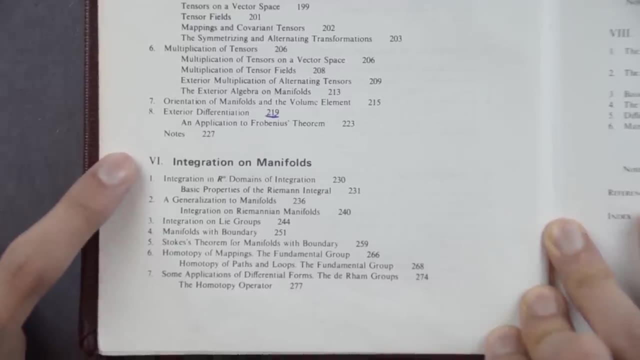 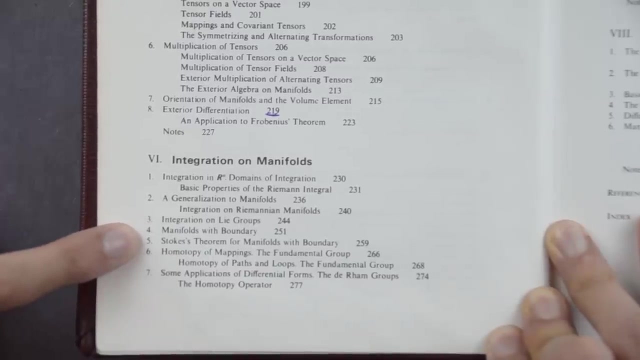 Next, it introduces the main technical tools, vector fields and tensor fields. The next chapter is Integration on Manifolds, which forms the heart of the book. There are two big theorems. Stokes's theorem, which is a vast generalization of the fundamental theorem of calculus. 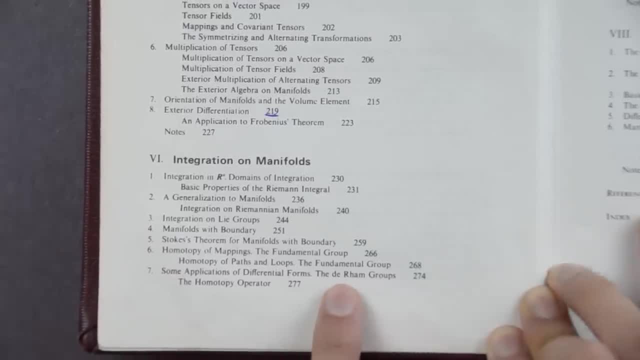 And Duram's theorem, which links topology and calculus in a stunning way. 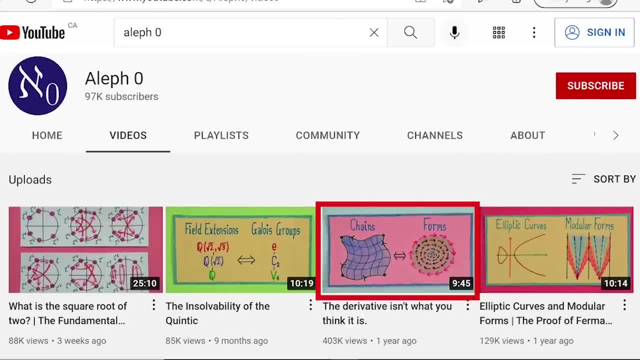 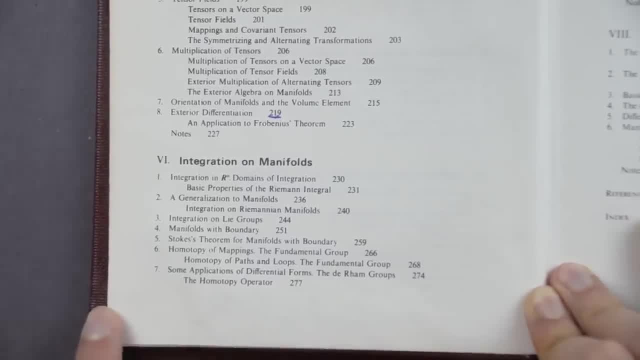 I've made a video about these topics if you'd like to see them in more detail. This part marks the end of the differential geometry portion of this book. 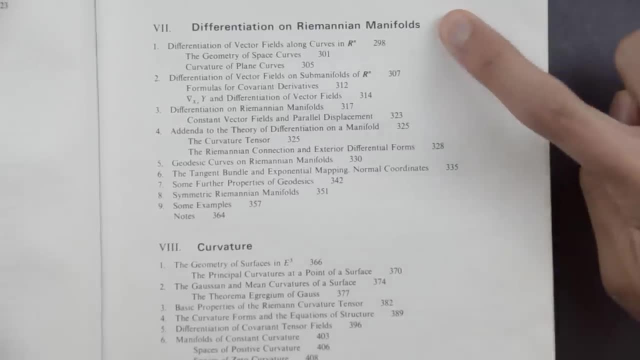 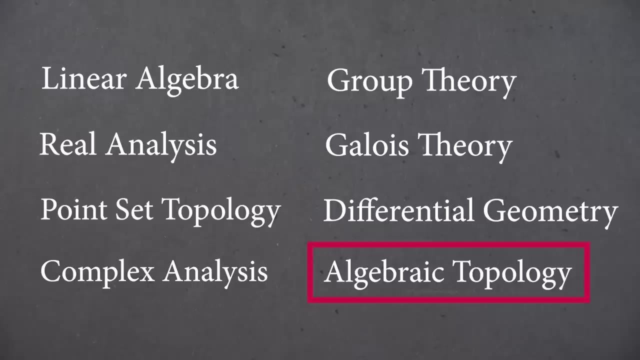 The second half of this book is about Riemannian Manifolds, which, roughly speaking, are curved surfaces with a notion of distance. Next up is Algebraic Topology. 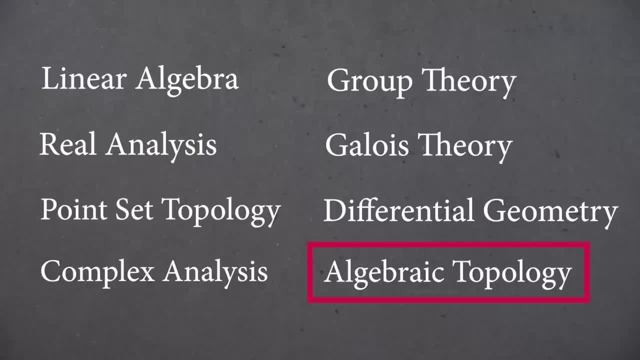 It's the study of how to use methods from group theory, to study questions from topology. 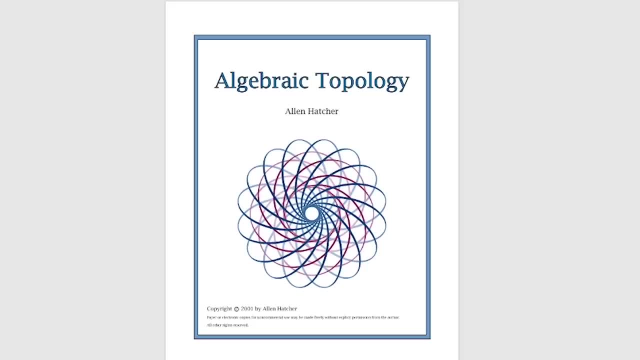 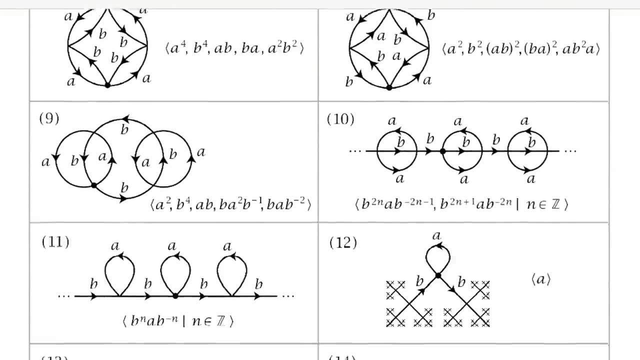 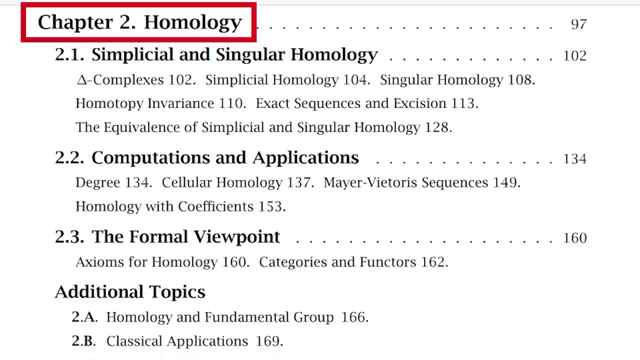 A wonderful book to learn this subject is the book Algebraic Topology by Alan Hatcher. The book is really, really wonderful. It has tons of pictures and tons of exercises. It has three parts. Homotopy. Homology. And cohomology. Which are the three main pillars of the subject. 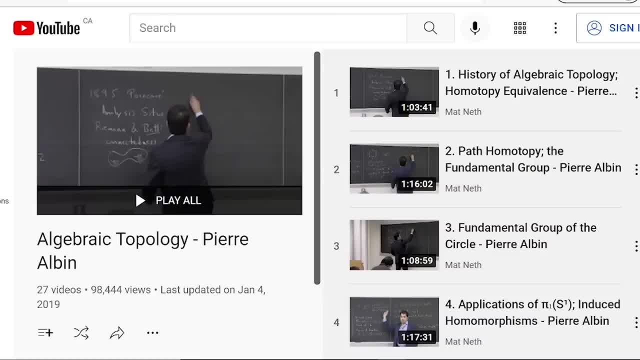 Another plus is that, Albin has made a lecture series that follows this book, pretty much chapter to chapter. 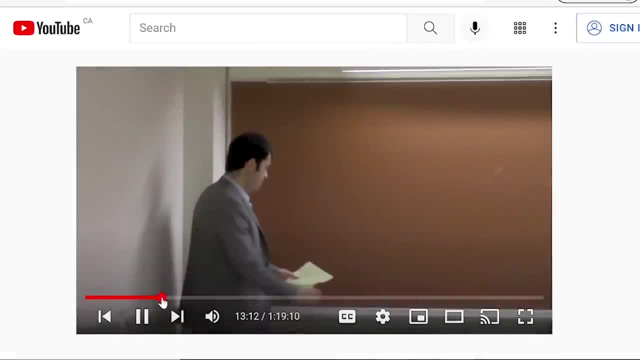 And he's made this lecture series freely available on YouTube. These lectures are also really great for understanding the material, and I've put the link in the description. That's all for now. 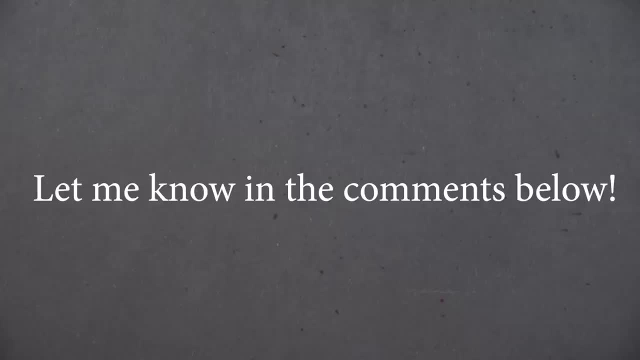 If you happen to know of any other resources for learning math that you found helpful, type them below in the comments and I'll be sure to add them in the description. Thanks a lot for watching, and I'll see you next video. Transcription by CastingWords 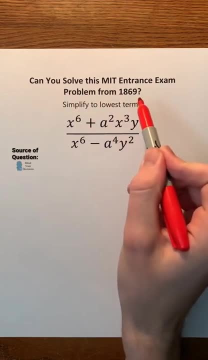 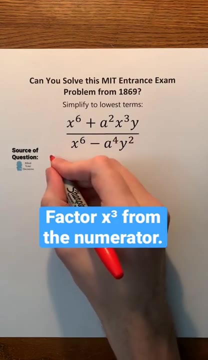 Can you solve this MIT entrance exam problem from 1869?? Simplify to lowest terms and we have this expression. First, we can factor x cubed from the numerator to end up with x cubed times the factor x cubed plus a squared y In the denominator. we can rewrite x to: 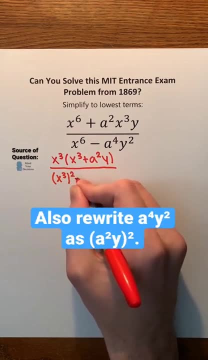 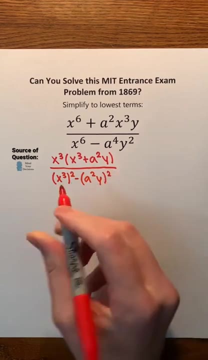 the power of 6 as x cubed to the power of 2.. We can also rewrite a to the 4th times y, squared as a to the power of 2 times y, and then raise the term to the power of 2.. Now 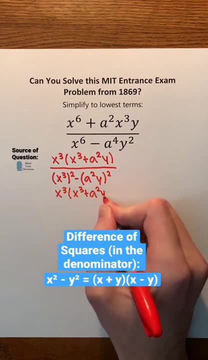 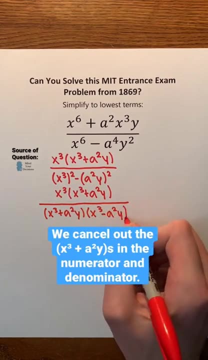 notice that we have a difference of squares in the denominator, so we can rewrite it as the factor x cubed plus a squared y times the factor x cubed minus a squared y. We can cancel out the x cubed plus a squared y's in the numerator and denominator, so we will. 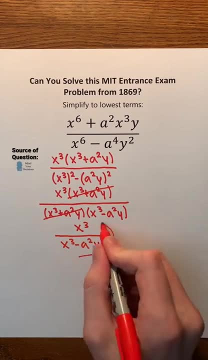 end up with x cubed over x cubed minus a squared y.